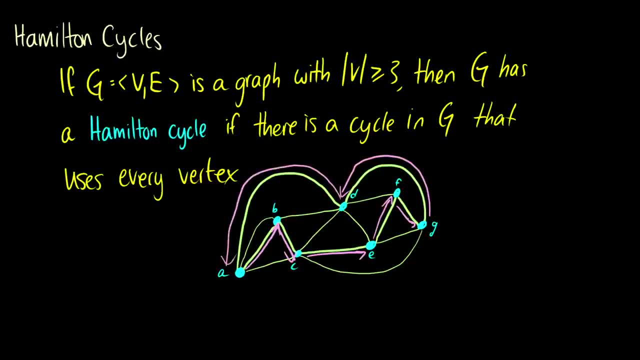 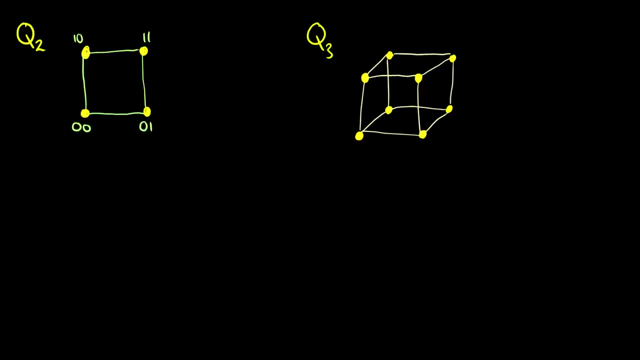 and let's loop all the way around back to A. So we've used A, B, C, E, F, G, D, A, So that's a Hamilton cycle, because we used each vertex exactly once. Okay, so here's a nice question, Can you? 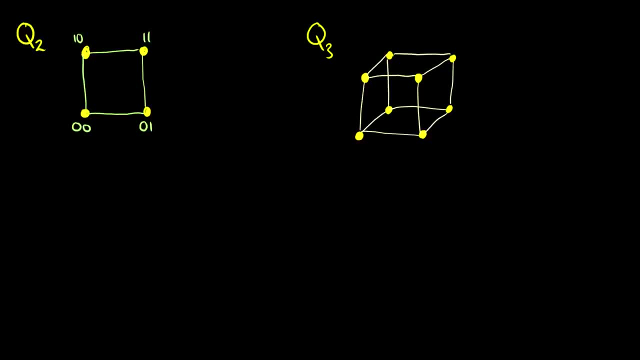 find a Hamilton cycle in a hypercube. Well, let's start at 0, 0.. Let's start right there. Okay, go 0, 1, 1, 1, 1, 0, 0, 0.. Oh, perfect, cool, really easy. What about in this? 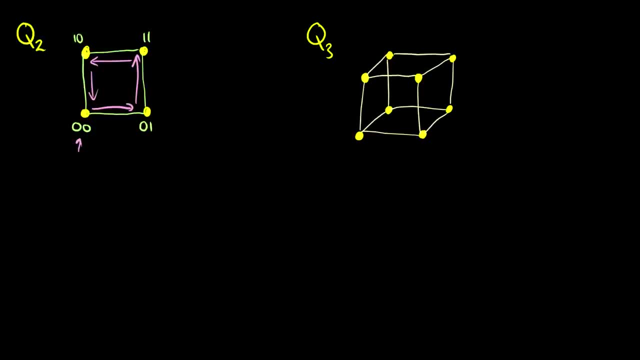 Q3? I need to check something quick. Okay, so Q3,. what we can do is we can sort of do the same thing. We can say, okay, let's do the front. So we sort of know how this works. We just do that. 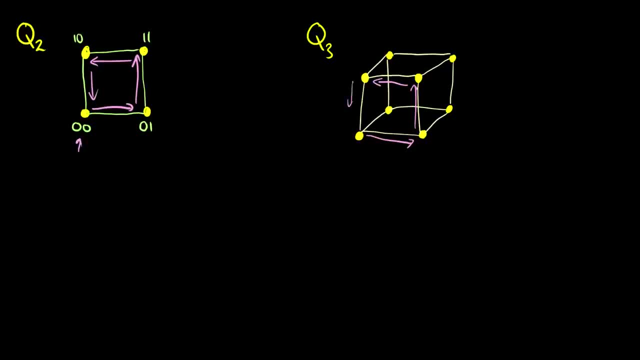 and when we had Q2, we went back down. But instead let's go back, then we'll go across, then we'll go down, then we'll go to the left here and then we'll go forward. And now we've. 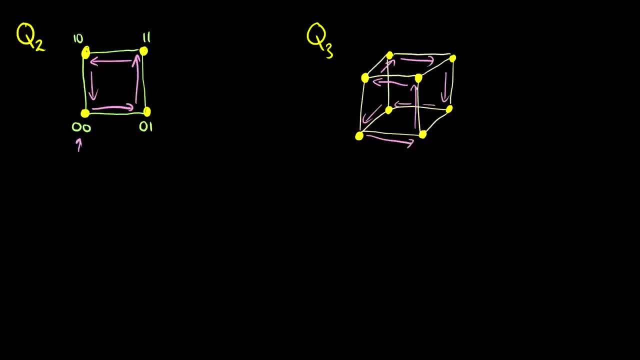 used each vertex exactly once, So this one's a little bit more complicated. So here's the question: Which hypercubes have Hamilton cycles? And if you check out trevtutorcom, discrete math 2, and look at the final exam there, there's a question that asks just that. But what I am going 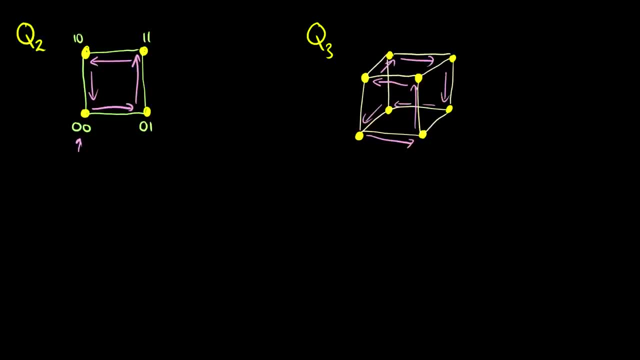 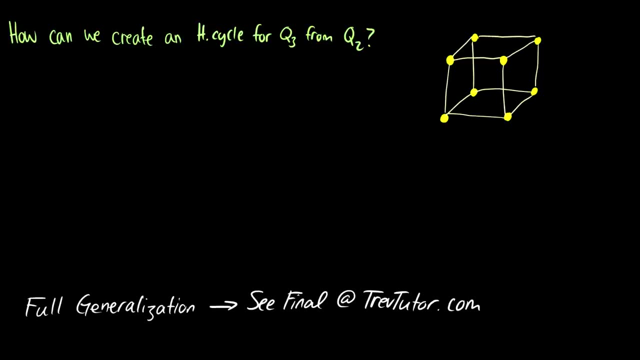 to do is lead you to a conclusion about hypergraphs or not hypergraphs, hypercubes. using this thing, How can we create a Hamilton cycle for Q3 from Q2? Okay, well, what we should do is split it up. 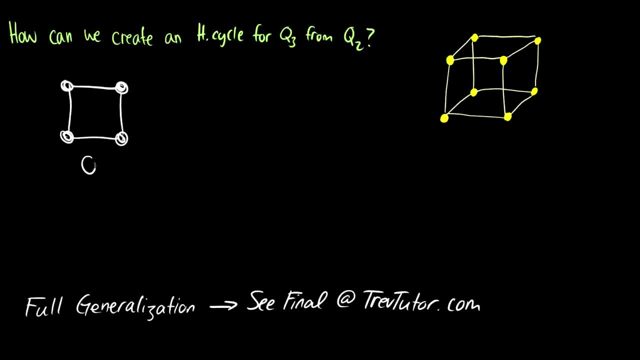 We'll call this one Q2 into 2 graphs. We're going to call this Q2.. And we're going to call this other one here Q2, prime. So we take a look, This front portion here is going to be Q2,. 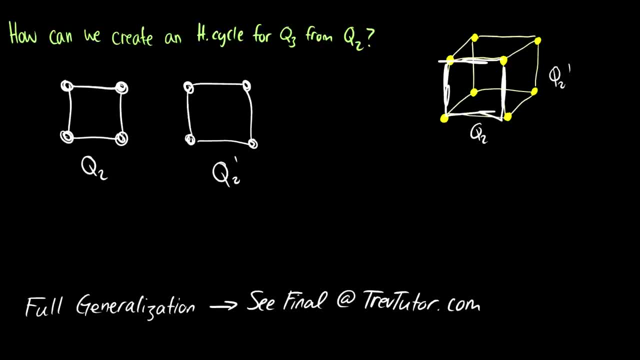 and the back portion will be Q2 prime. So we have a Hamilton cycle for it. So they're, these squares that sort of go in a counterclockwise direction. They can go clockwise if you want. Here's what we're going to do to create a Hamilton cycle. 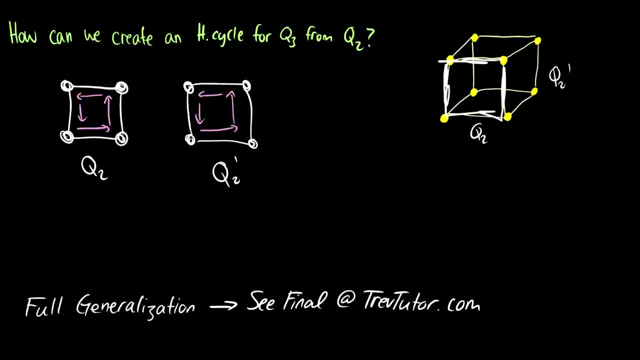 Well, we're going to take Q2.. So we're going to go from A to B to C to D. So what we're going to do is we're going to remove this last edge that goes back to A. We're not going to take that. 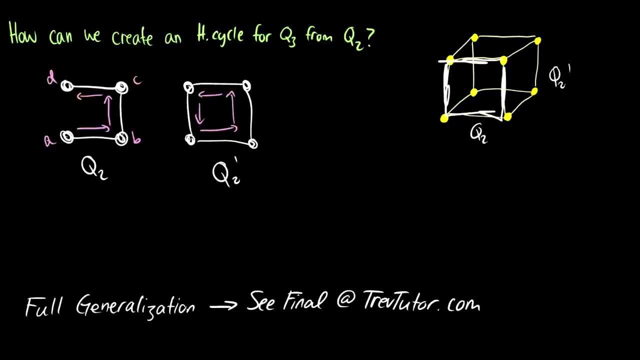 So we're going to do that, We're going to remove D to A, So we go from A, B, C, D. But then what we know is that, well, all of these points connect to their counterparts, So we have those two connecting. 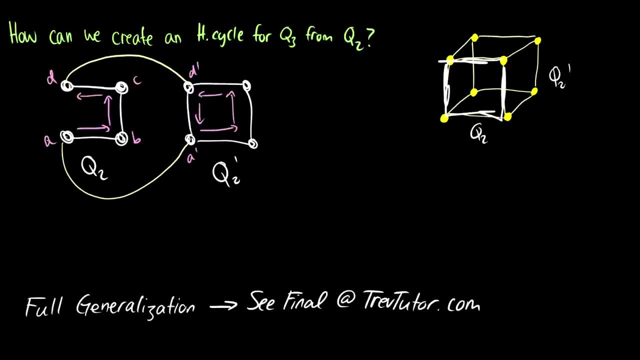 which we'll label these D' and A' We have B' and C' I'm not going to draw those connections because they're a little bit difficult to overlap and make it look nice, So we'll just forgo those. And so what we're going to do is we're going to take Q2,. 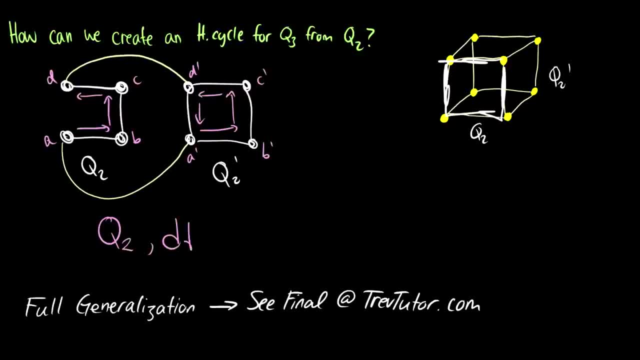 and then we're going to take this D D' path, because we got to the end of our trail here And we're just going to take it over to the back. Then what we're going to do is we're going to take the Hamilton cycle for Q2.. 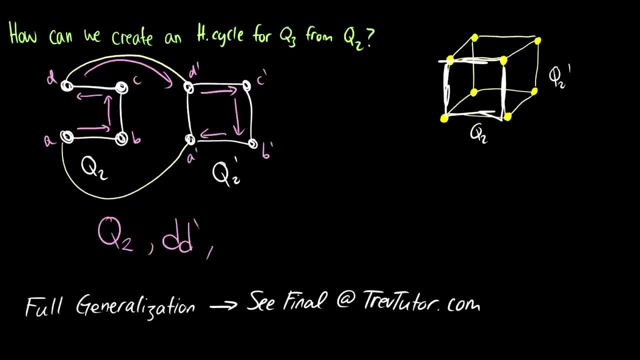 We're going to do it in reverse. So, instead of going from A to D, we're going to go from D to A in the back. So we're going from D' to A' So we're going to take this Q2' trail or path. sorry, 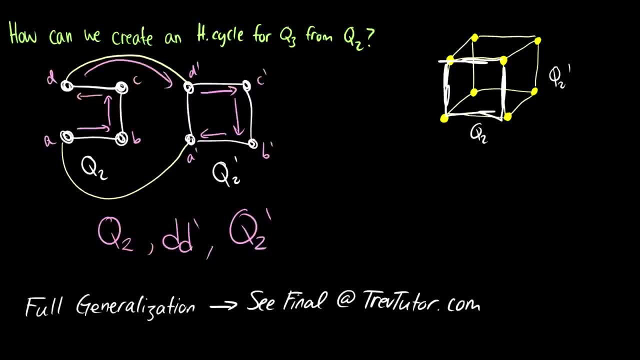 Okay, then what do you think we do now? Well, we take A' back to A, So we take this A'A, and now we have a Hamilton cycle. So we sort of broke up Q2 into two parts. We almost completed the cycle for both of them. 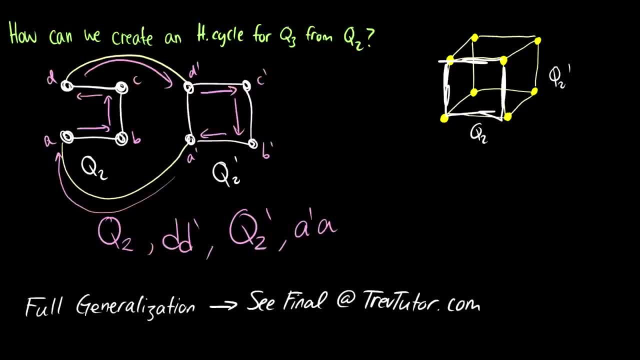 But we connected them right before the last path And that creates a Hamilton cycle. You can do this for Q4 by taking Q3 and Q3' along with two extra edges, And those two extra edges will be used to connect Q3 to Q3' and Q3' back to Q3. 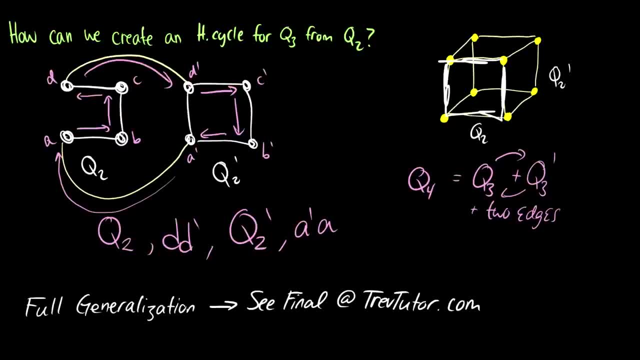 And you can connect them to Q3. And you can connect them to Q3' right before the last path, And we're going to take A' D And that creates a Hamilton cycle. continue this on and on. So what I challenge you to do at home is to figure out a Hamilton. 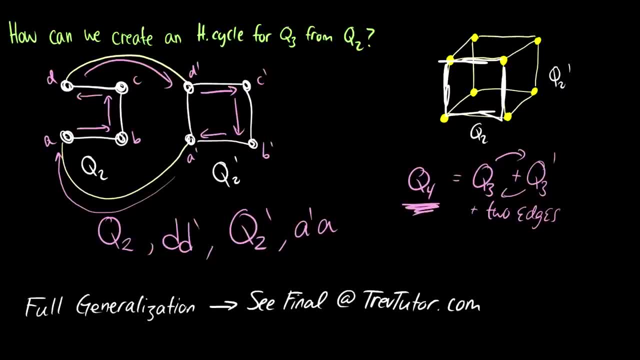 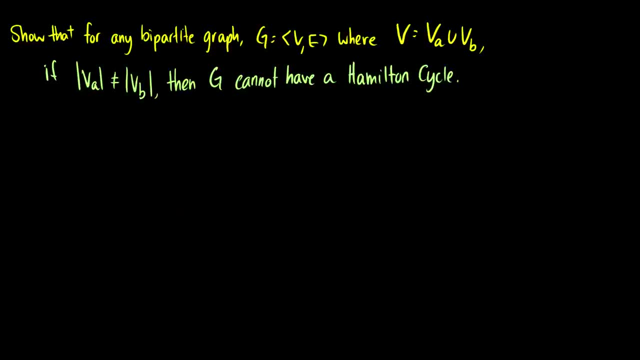 cycle for Q4.. So if you can do that, that is awesome. But we should probably talk about one more thing, about Hamilton cycles. here I know it's kind of short. The proofs for Hamilton cycles are fairly difficult and you generally wouldn't need to know how to. 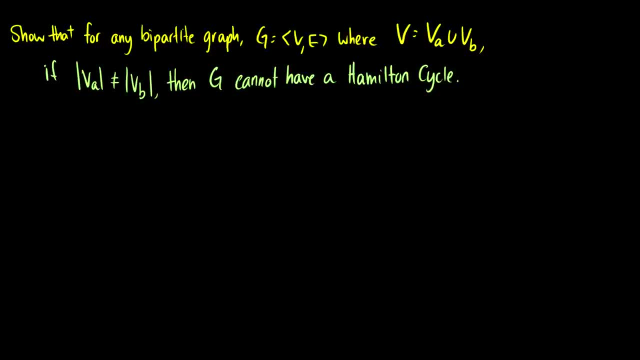 prove them in an introductory discrete math course. That's more of a graph theory course, you know, proof-heavy course. So we're going to forgo the proof and instead we're going to take a look at bipartite graphs. So this is a nice trick that people can throw on a. 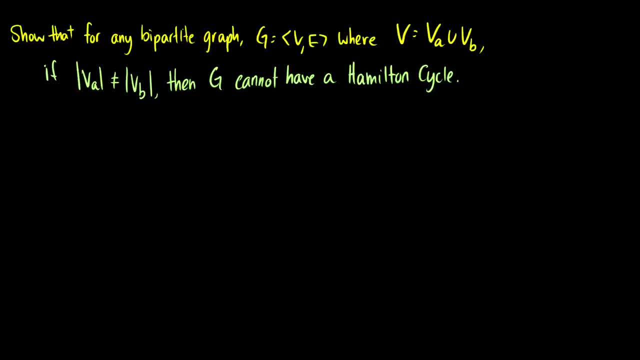 final exam They can say: here's a graph, Does it contain a Hamilton cycle? And Hamilton cycles are very hard to find, So you need tricks to sort of prove them in an introductory breakup graphs. And a good thing to do is check: is the graph bipartite? Because if 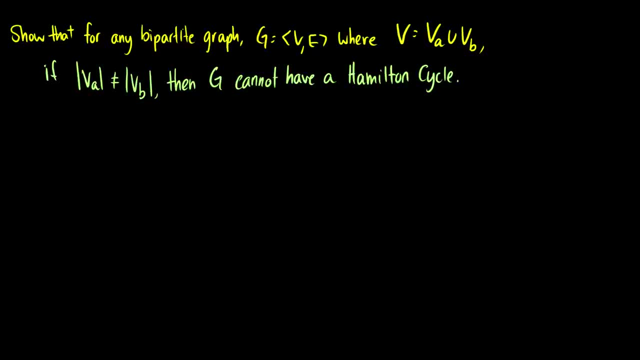 it is. we have this lovely theorem here: If we have a bipartite graph where V is split up into two different parts, if VA and VB don't have the same amount of vertices, then we can't possibly have a Hamilton cycle. So let's take a look at what happens when we 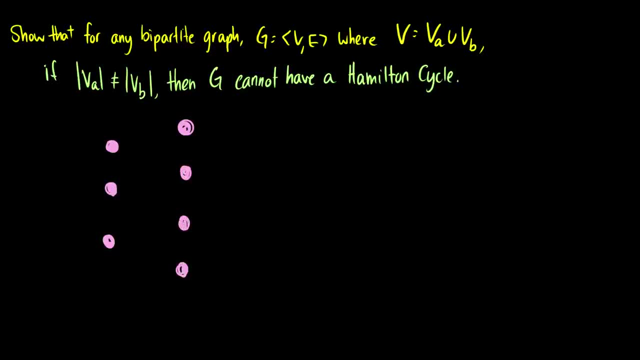 have a Hamilton cycle where our VA and our VB are not equal in size. So we're going to do two cases. One is where we start in VB and the other case is where we start in VA. So we want a Hamilton cycle, so it has to connect all of the vertices exactly once. 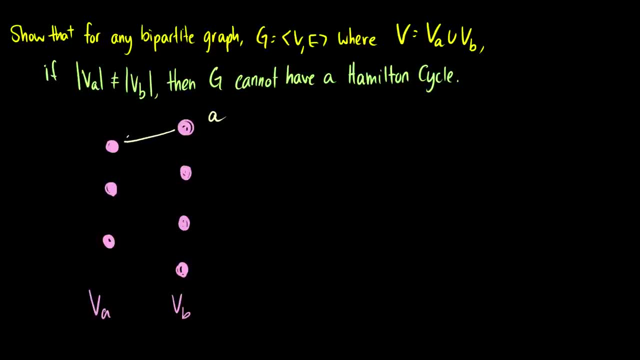 So here's what happens: We go from VB to VA, Then we go from VA to VB, If we just let it go back and forth- but then what happens is that when we get to this last in VA, we still have to use VB. So we have to use this last vertex in VB. The problem: 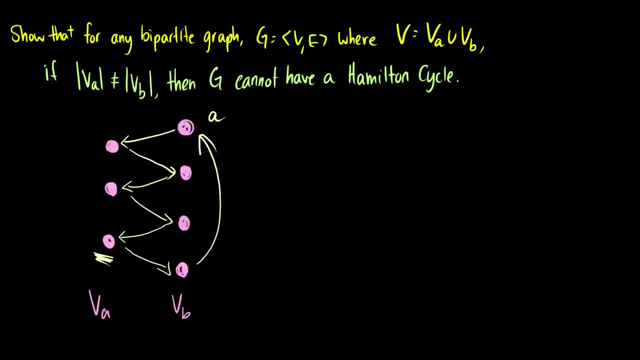 is that now we have to go directly back to A, but because the graph is bipartite, we can't do that. We have to re-use a vertex in VA. So instead we say: no, that can't happen. bipartite graphs cannot have a Hamilton cycle, in this case, when we start in the bigger side. 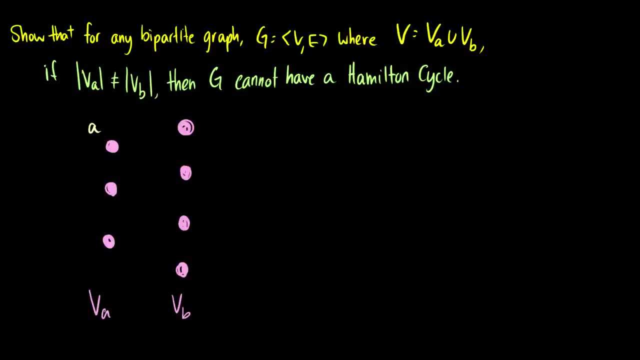 But what if we start in the smaller side here? Then surely we might have some luck. Okay, so we go from VA to VB. We go back and forth. Now we run into a problem here, because we've done as much as we can and now we have to go back to VA to finish the cycle. The problem is that we're 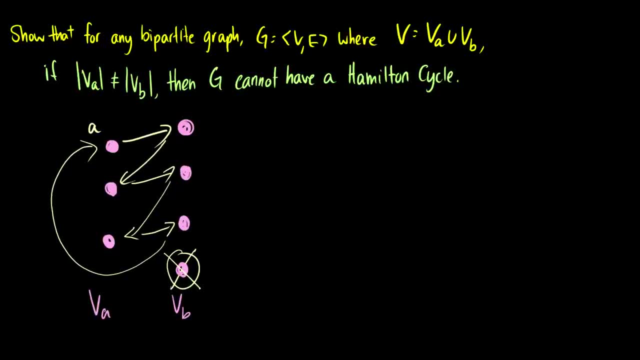 still missing this one vertex in VB that we can't get to because, well, after we go back to A we'd have to go to VB, but by then the cycle's complete, so we can't have a Hamilton cycle. So we've just proven the two cases that are possible and we've proven that we can't have. 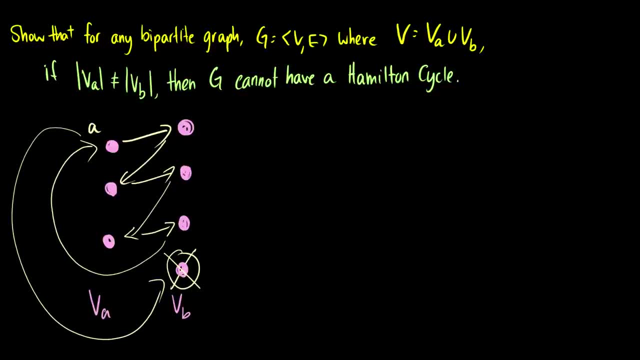 a Hamilton cycle then. So there you have it. If the two sizes of the bipartite graph are not even, then they can't have a Hamilton cycle. So here's a question: Can K43 have a Hamilton cycle? And the answer straight away, when you see: 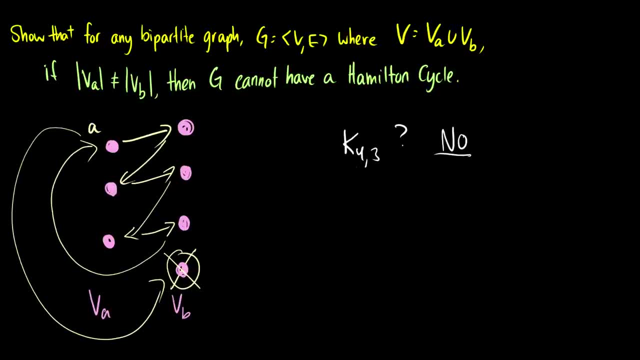 it is no, it can't, because this one side is bigger than the other. Can K7171 have a Hamilton cycle? And the answer is yes, it can, because, well, they both have 71 vertices. so we're good. Now 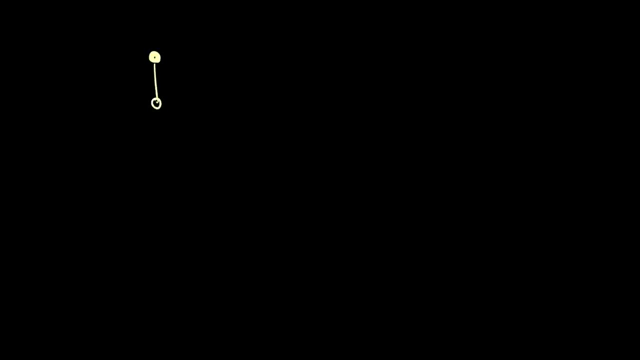 what sort of question can they give you with a graph? Well, here's a nice bipartite graph that you don't necessarily see too much in textbooks and unless you talked in class about this or lectured, you generally don't see this immediately as a bipartite graph. But this is a bipartite. 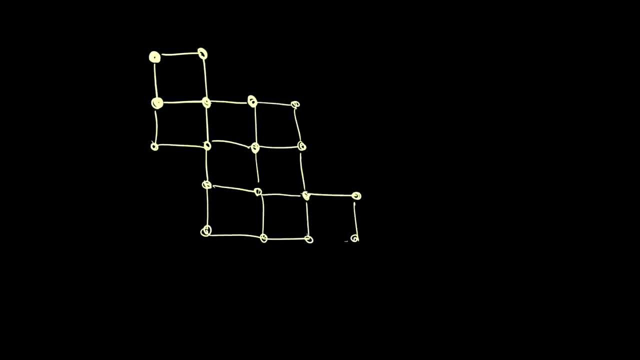 graph. So here's the question: Does this graph have a Hamilton cycle? And what you have to do is take a look and you have to figure out. okay, we need to label these ones and twos and we need to see how many are going to be in v1 and how many are going to be in 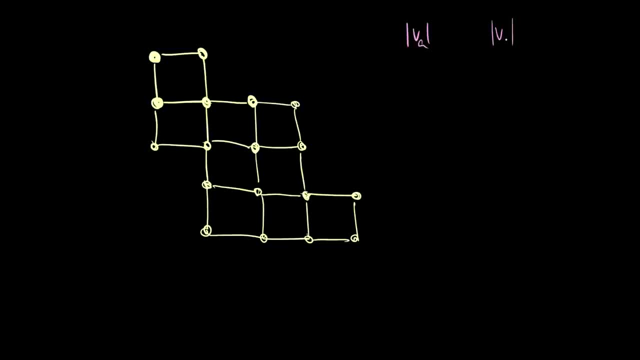 v2.. So let's just call this va and vb for consistency. So we're going to alternate, So we're going to have a bb a, b a, b a, b a. We need to make sure we don't get any. 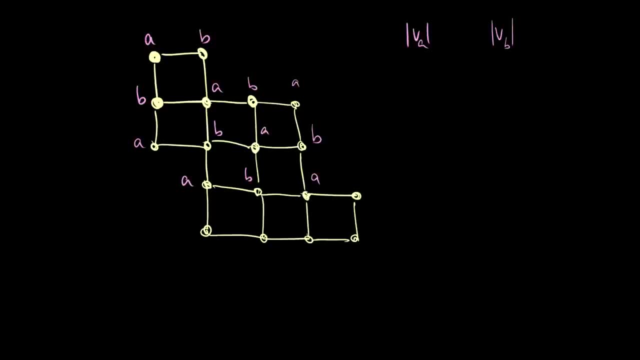 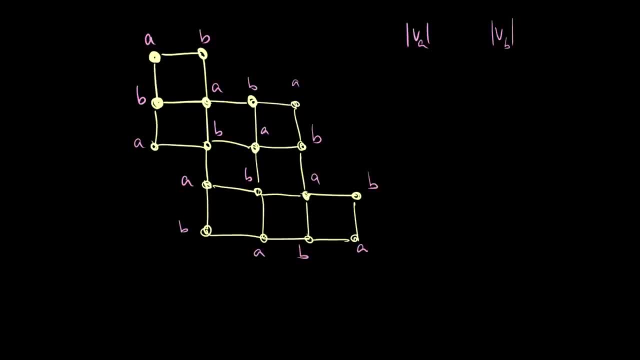 one, two, three, four, five, six, seven, eight nine a's. How many b's? One, two, three, four, five, six, seven, eight, nine b's. So here's the question: Does this graph have a Hamilton cycle? 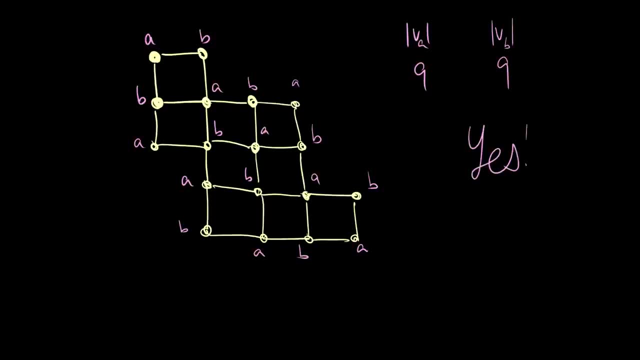 And the answer is yes, because va is equal to vb. What is the Hamilton cycle? It could be anything. Let's try to construct one. Let's start at this a up here. Let's go right down, right right down down. We'll just go along the edges and we'll see what happens here. 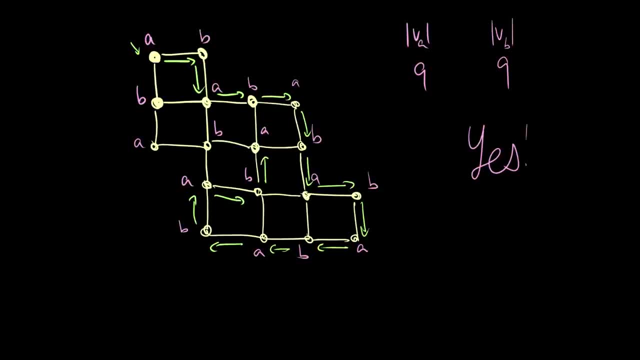 So, okay, we need to hit this b here. We need to go up, go to the left, left up. Okay, there we go. There's a nice Hamilton cycle. They can be hard to find. This one was generally easy to find. 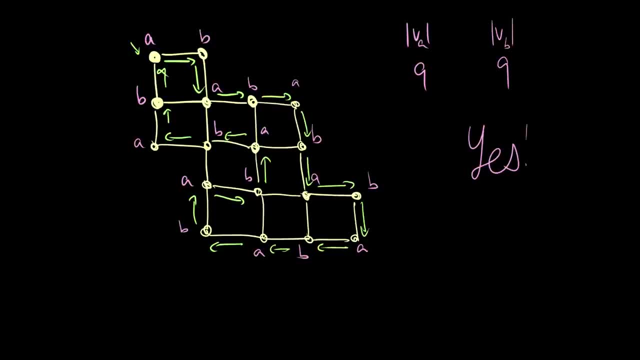 but they can be difficult, So hopefully you don't have to point one out, because that can get tricky. But that was basically the quick and dirty introduction to Hamilton cycles. If you want really rigorous proofs of this stuff, definitely read them in your textbook or online. There's tons. Perhaps in the future 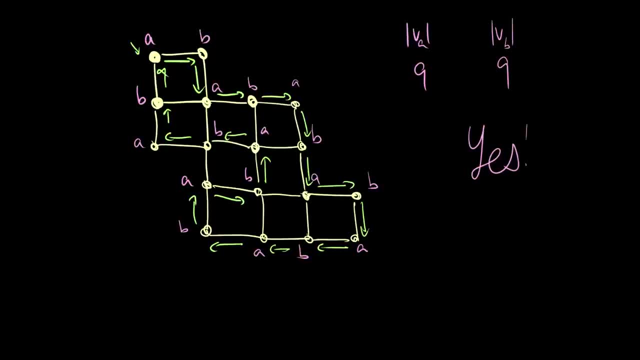 I'll do a proof heavy if I ever do a graph theory course, but that's not really in the works right now. I have other projects like linear algebra and pre-calculus to get through first, So we'll see how that goes. But if you have any questions, leave them in the comments below.